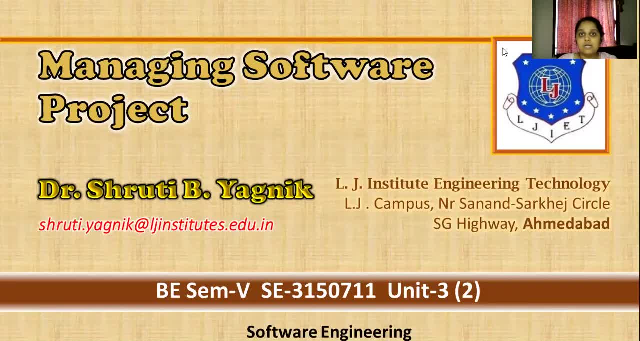 how the other stakeholders they are working collaboratively through W5HH principles. We also know about the four P's of product management or development. We also know about how risk is to be handled in software projects. We also discussed that your project always needs a particular schedule and, based on that schedule, 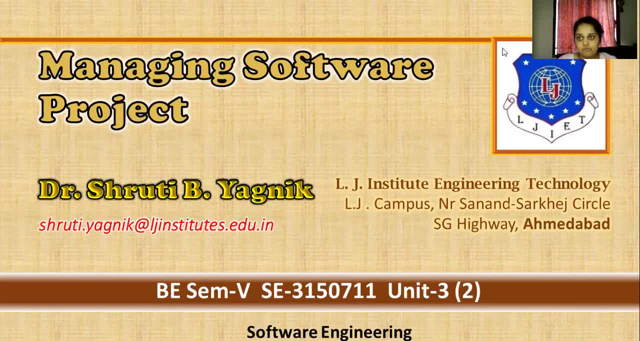 you are supposed to develop the project so that you come to know how much you have progressed, how many milestones are yet to be covered. We also have seen that you are breaking down your tasks, you are compartmentalizing them or dividing your works into subtasks, and you 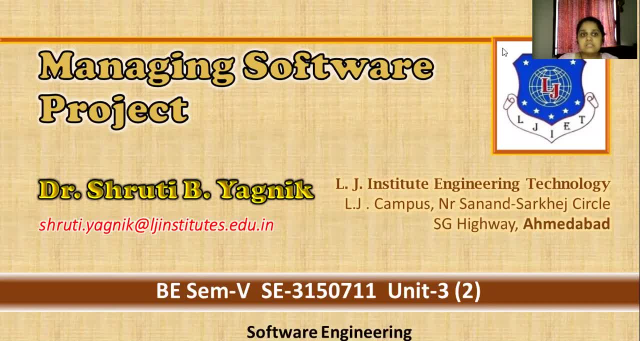 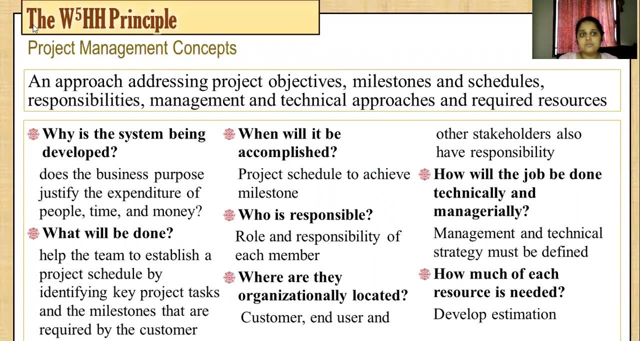 are plotting them in a Gantt chart, and all these things will help you to manage the software projects. So let us have a brief about what we saw in the previous lecture, The previous lecture. we have seen the W5HH principle, which is a project management concept. 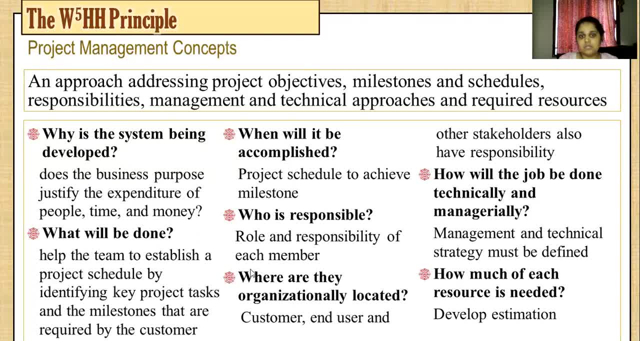 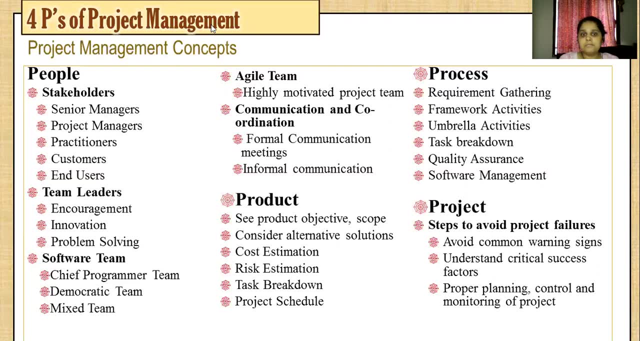 And we saw how 5Ws 1,, 2,, 3, 4 and 5Ws and HHH are helping you to have this development principle. Next we saw is the four P's of project management, which included people, product, process and project. 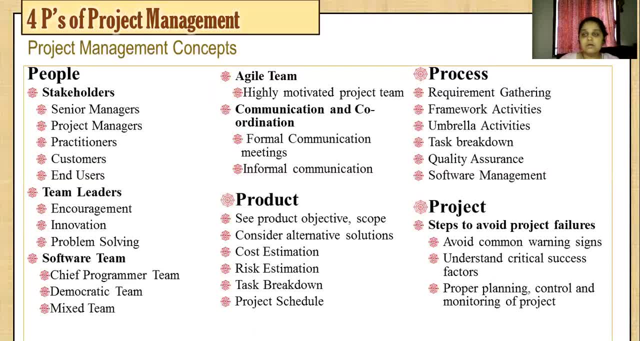 We saw who are the stakeholders, What a team consists of, what type of team structures we were promoting, what an agile team is and what are the ways in which this team works. We saw what a product would be. we saw what is handled while you are making a product. 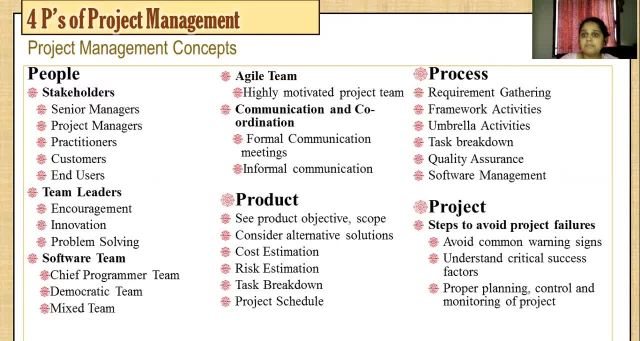 We saw how you are working towards the project making. you are seeing the processes in detail. We also saw how you are supposed to tackle a project so that it doesn't fail. So we saw the steps to avoid project failures by having a proper tracking and control. 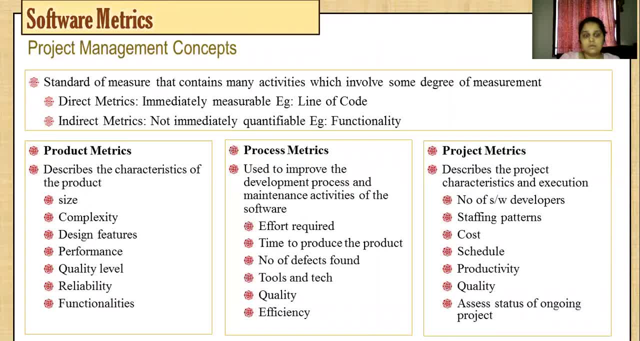 This was the team structure that we saw. OK, today we shall move on to software metrics. Now, what are software metrics actually? So, before we move on to software metrics, let us first know What software metrics actually mean. Now, metrics are nothing but a simple or you can say: let us say, for example, you want to measure weight. 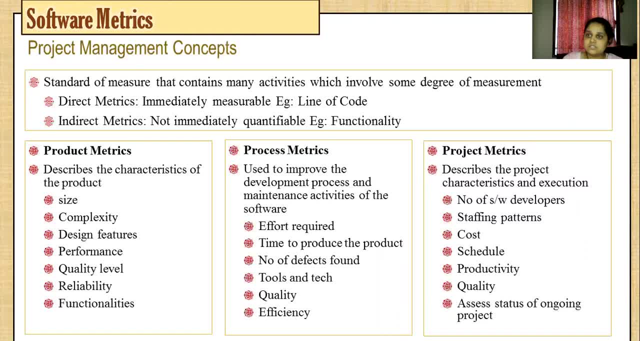 So if you want to measure weight, you measure it in kgs. If you want to measure height, you measure in centimeters or inch or feet. If you want to measure distance, you measure in kilometers. OK, now I want to measure my software. 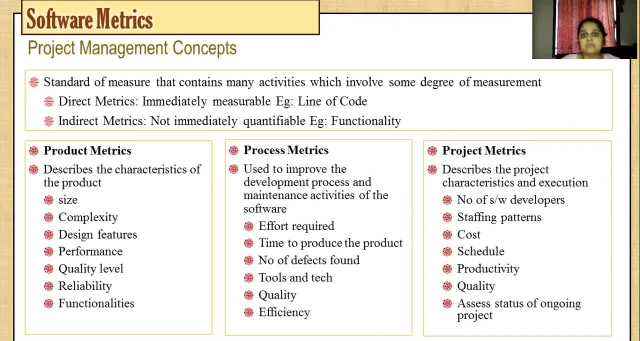 So if I want to measure the software, then we need something called as software metrics. Now, this software metrics is nothing but a standard of measurement of a software where there are many, many activities happening, And we want to measure those activities in order to find out the total estimates of effort or estimate of the size of the project. 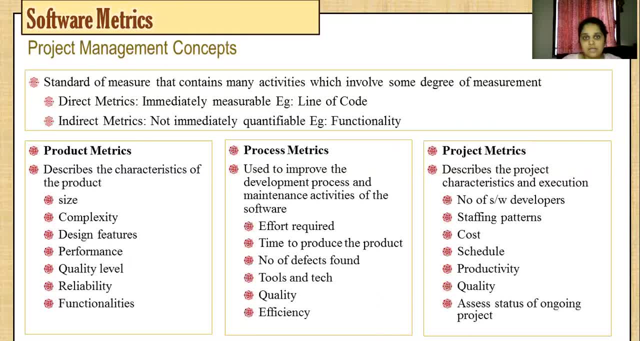 So if we don't measure the software, we will not be able to predict how much effort is to be used in the software, how much budget should be included, how much long should the schedule be? how much long duration will it take for the project to be completed? 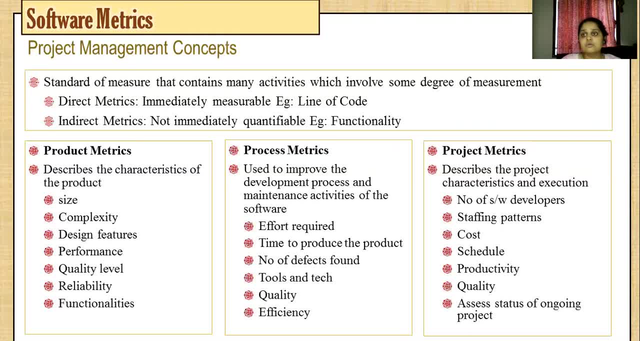 So, due to these reasons, it is very, very necessary to measure the software, and software metrics comes to your help in this case. Let us take a simple example. if a manager is managing the software, what is he going to check? He is going to check for reliability. he is going to check for size of the software. he is 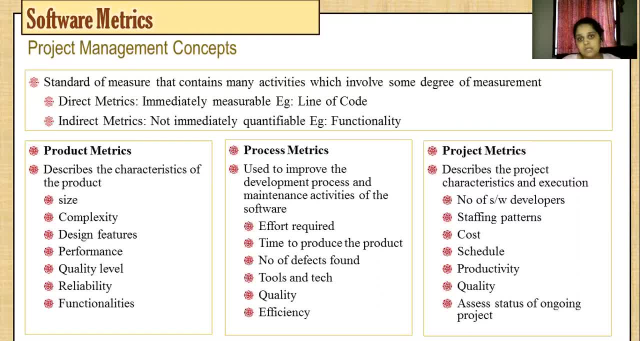 going to check what is, what could be the completion time. he will check what could be the efforts that we need to put in, how much resource we need to add, resource in form of manpower, resource in terms of money. Then, if you want to keep, 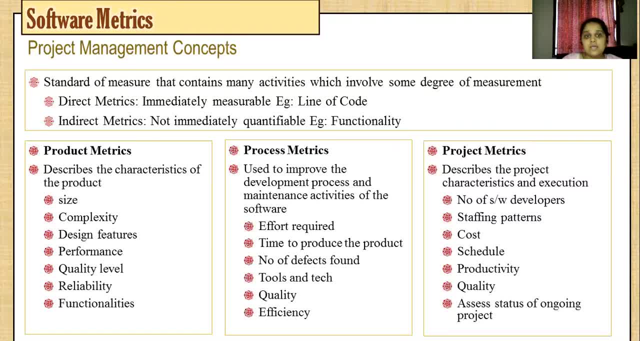 a check of all these things. you need to check the function or functionalities that you are implementing in your project, and you also need to check the size of the project. So these are the two basic things which you need to check, and software metrics will help you to do these things. It will help you to predict. 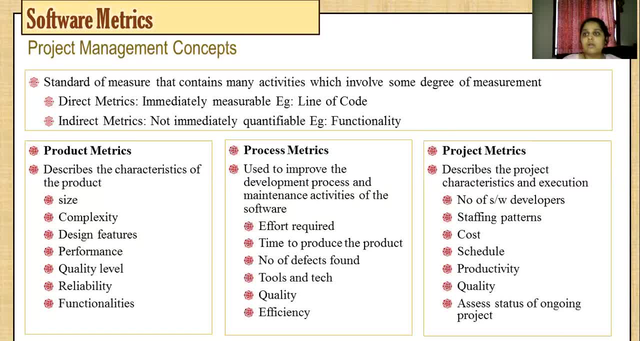 the size of your software by calculating the overall code that you are going to make and by the functionalities that you are going to to the client. okay, so let us see the definition of project or software matrix. software matrix is nothing but a standard of measure. so it is nothing but. 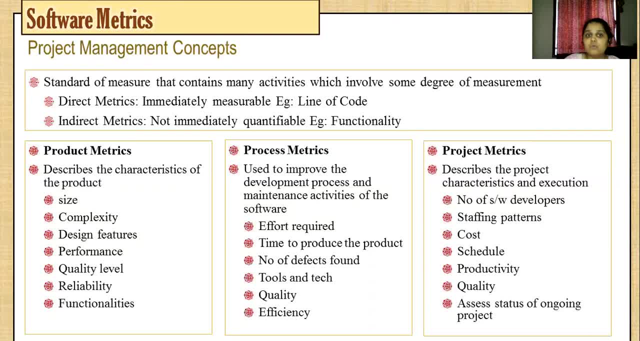 a kind of measurement, and this measurement is doing what this measurement contains? many activities which involves some degree of measurement. okay, so what I am doing is there are small, short, short measurements which you are taking at regular intervals, you are combining them and you are creating one particular measure. so this measure is nothing but a. 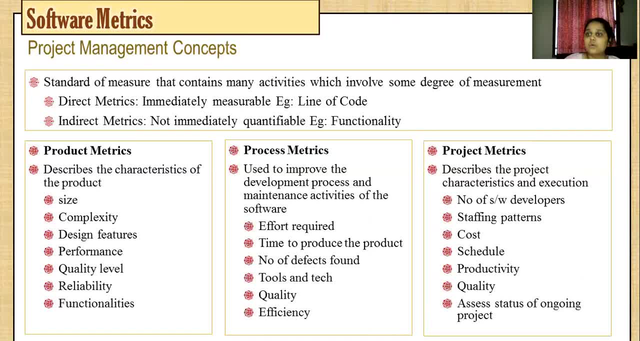 software matrix, and this matrix is going to help you to find out what is the size of your software. okay, okay now. metrics are of two types. first is direct matrix and indirect matrix. now, direct matrix is something which can directly be calculated through your perfect editor. so I am saying that. 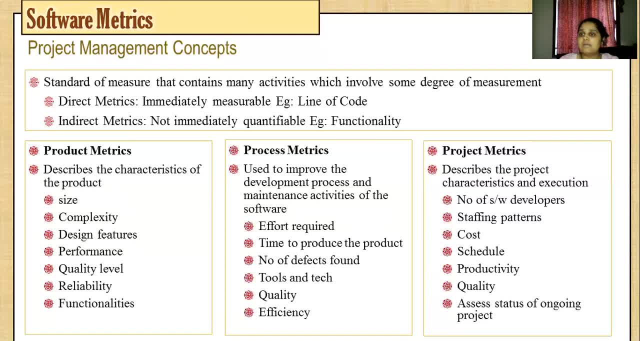 if I say the student has got 53 marks, so 53 is something, well, which can be easily calculated, or it is a number so it can be measured easily. okay, so that is a direct matrix. the example of direct matrix is line of code. now, line of code means how many lines of codes you are writing in your product, or 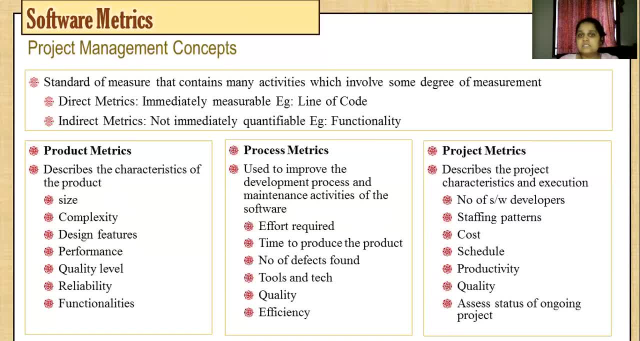 of your program. So if you are writing a simple program, be it C, be it Java, be it C++, be it Python, be it any language, So number of lines that you are writing in your editor is your line of code. So line of code is something which can 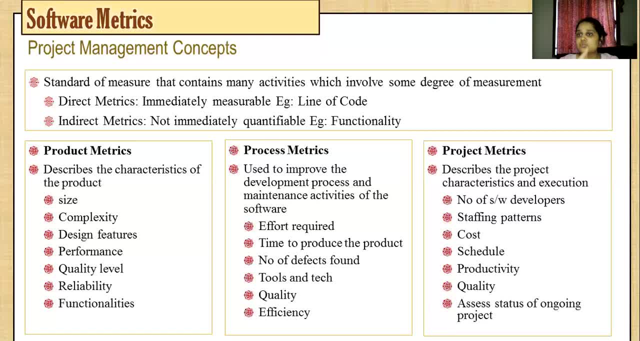 be immediately measured. Okay, in some editors you have the line numbers written in just on the start, that is, on the left hand side. So that is a direct matrix. and second is indirect matrix. Indirect matrix is not actually a number, Okay, but it is not immediately measurable. So let us take 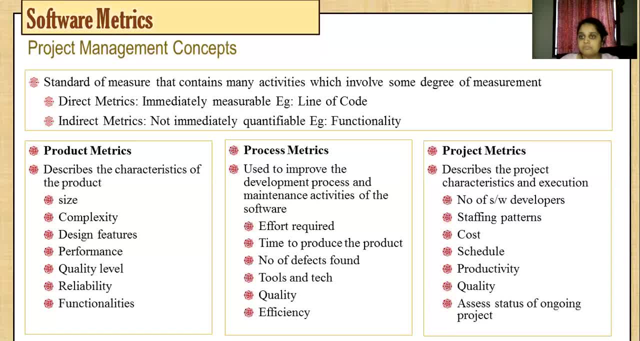 an example of indirect matrix is functionality. Now, functionality is what kind of features you are implementing in the system. We don't say I'm implementing five features. We don't say I'm implementing six features, Because each and every feature has some features maybe may. 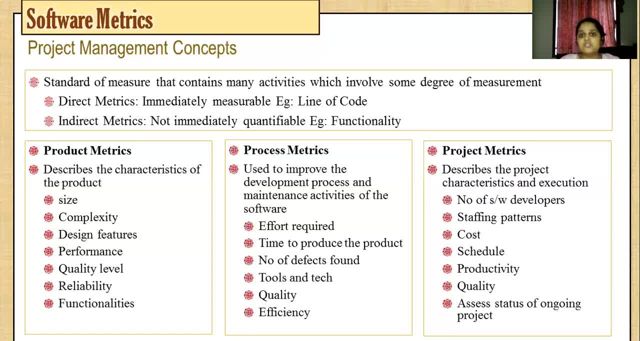 require a very long time to be implemented. Some features may require very short time to be completed. So you can't consider both these functionalities as a, as you know, as equal. So if you are not considering them as equal, you cannot number them, that there are five functionalities or six functionalities. 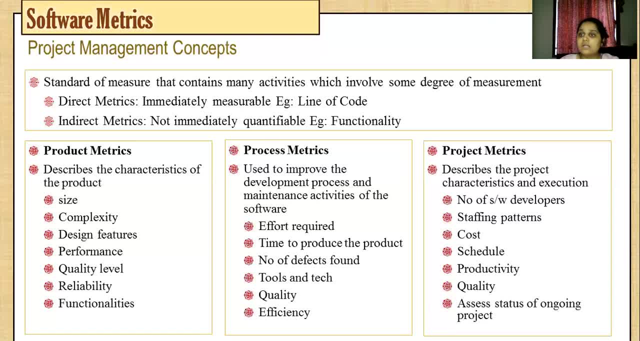 as they are unequal. In that case, you are not immediately measuring them and it is an indirect matrix, So you need to measure how many number of lines of code you have through direct matrix and how many functionalities you are delivering with each and every importance of with importance. 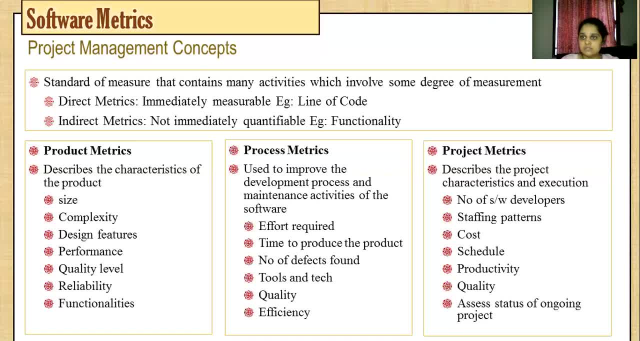 of each and every functionality through the indirect matrix. Okay, So now let us move on to product matrix. Product matrix is nothing but it describes the characteristics of the product. So product is nothing but the thing that you are going to see. So what is the characteristic of the product that is being delivered? 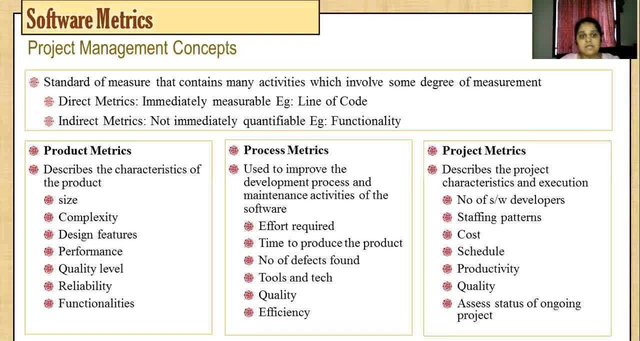 to the customer. So you can see that product matrix is measures, measure related to product measuring activities which are related to the product. So product matrix is having size as a characteristic because when your product is delivered you will see how many lines of codes you have done, how many functionalities you have given. so 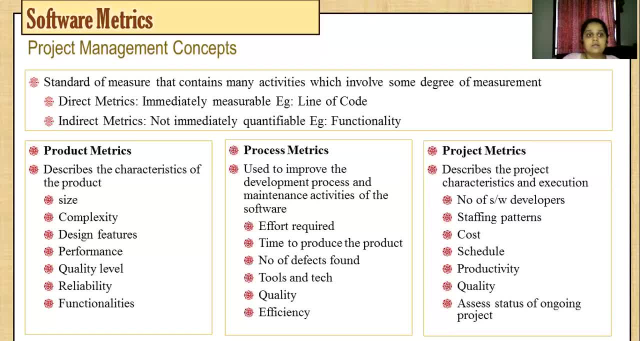 that will decide the size of your project. then. then you have complexity. How complex is the product that you are delivering? What are the design features that you are including in your product? What kind of performance your product is giving? is the quality level, quality assurance certificate given to your product? is their product? 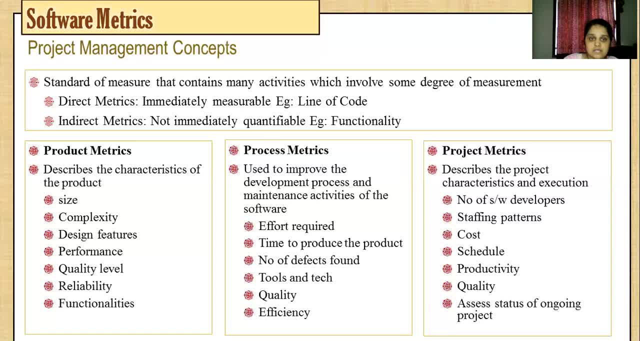 reliable and are all the functionalities which are asked by the user delivered in the product? So all this is going to describe all these things are described by the product metrics. next we move on to process metrics. now, product metrics. You have these many criterias now. after studying all these various 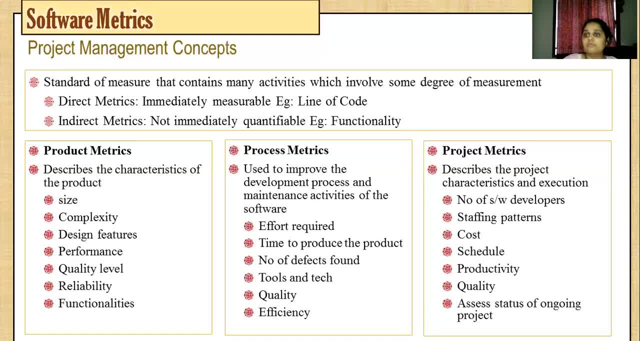 criterias, you can decide what kind of process you will follow to get the following product. Okay, so if you want such a product which has all these criterias very satisfactorily satisfied, then what kind of process you need to follow in order to get a good product, so that you can see here. 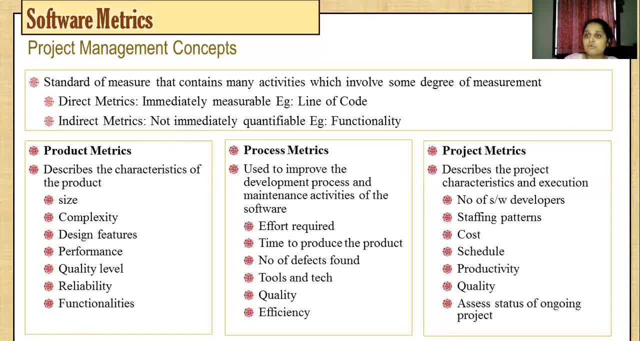 Okay, so process is nothing, but it is used to improve the development process And maintenance activity of a software. Okay, so you can say: this is something which you are giving as an after service or something which is in the life cycle of the software development. 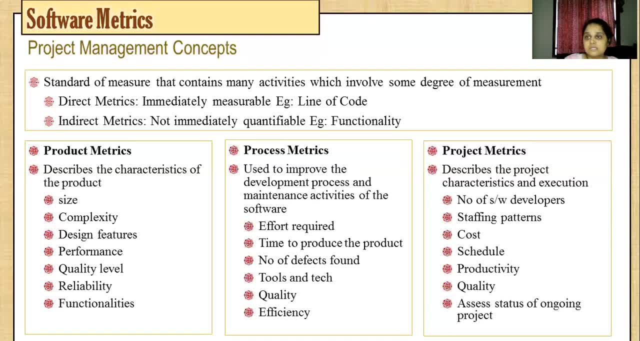 So first is if your process metrics will tell you about what effort you are, you need actually to put into software development. it will tell you about the time required to develop the product. It will tell you about number of defects which are found. It will tell you about certain tools and techniques. 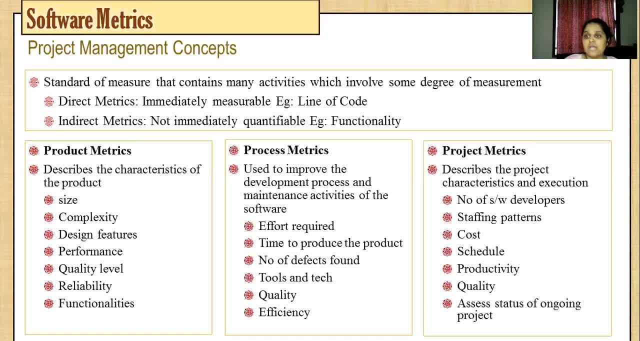 It may be possible that you are not aware of certain tools or techniques to develop something, So you require some time to learn them and incorporating the new software that you are making, You also need to assure quality and you need to check for efficiency. So if your process is good, your product has to be good. 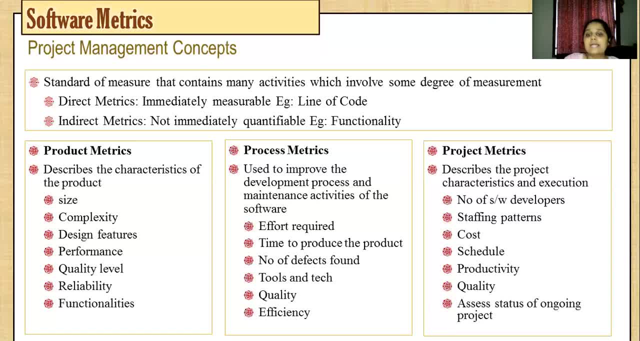 Otherwise, no, Okay. and next and last is project metrics. project metrics describes the characteristics of an execution of your project, So it will tell you how your project should be executed with how many number of developers. if you require 10 developers and you are hiring, say, 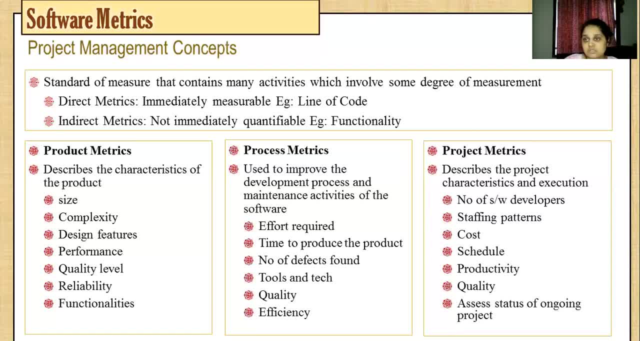 12 to 13 developers. you are wasting your resources. How many resources? first, you are wasting your manpower. second, you are wasting your budget. Okay, So these things are, you can say, very useful for project execution can. next is staffing pattern. What kind of a staffing pattern you are following? whether it is Chief, 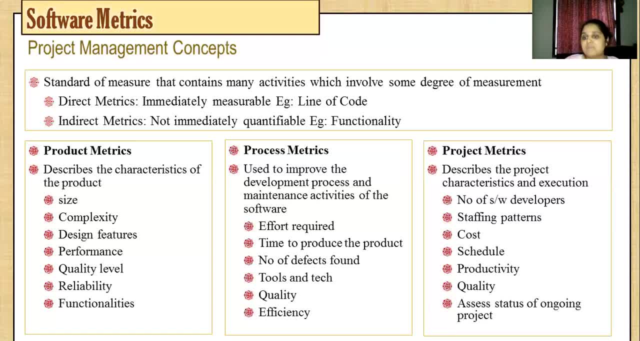 Programmer, whether it is Democratic, whether it is mixed, whether the team members are gelling well, whether they are communicating properly with each other. Next is you are dealing with cost. cost is nothing, but what is the budget that you have allotted to this particular project? 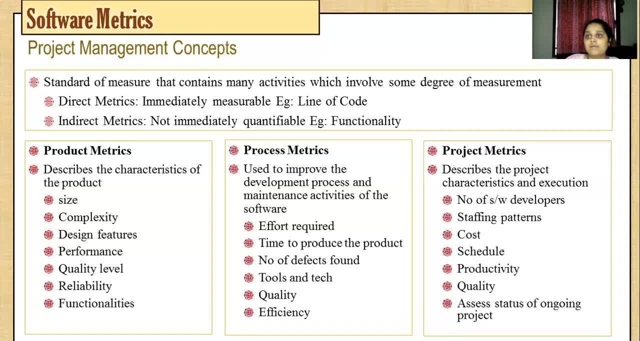 What is the schedule you are going to follow, whether the project is Spanning in one week or 15 days, or one month or six months or an yearly project. So schedule is decided, productivity is decided, that How this software will be useful and how faster you will be able to give. 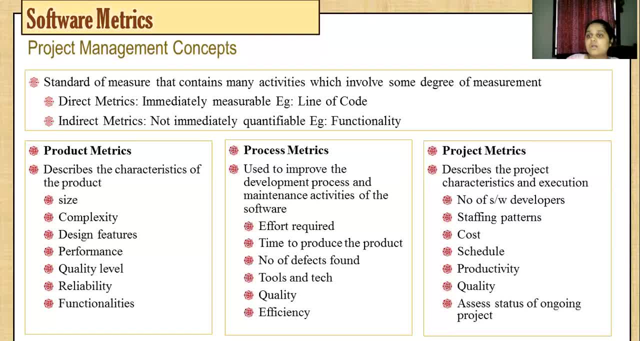 it with, with better quality. and what is the current status where you are in your whole schedule, How many milestones you have covered and how many milestones are yet to be covered. So these, this is what software metrics are. we shall now move on to how you are measuring software cost and effort. 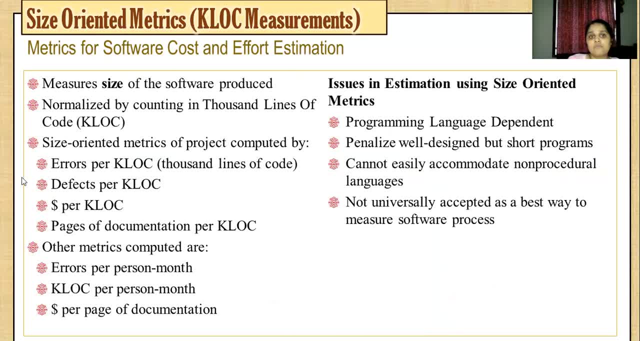 Okay, so metrics for software: cost and effort estimation. We are estimating the cost and efforts, So first is the size-oriented metrics, second is function-oriented metrics, Next is object-oriented metrics and use case-oriented metrics. We will cover all these in details in the next lecture. 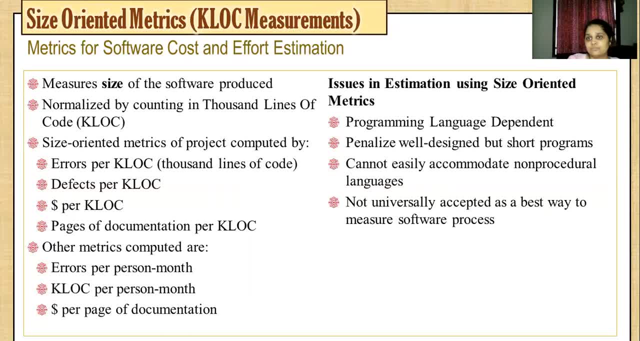 This is all for today, Thank you, Thank you.